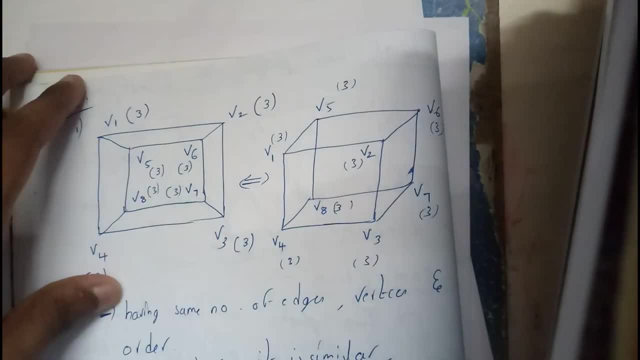 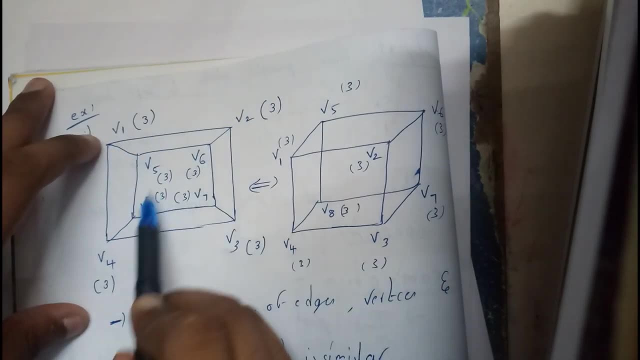 But these both are isomorphic, Whereas if they gave some diagram and they asked you to prove it. So initially take this as V1, V2,, V3, V4, V5,, V6,, V7,, V8.. It's all up to. 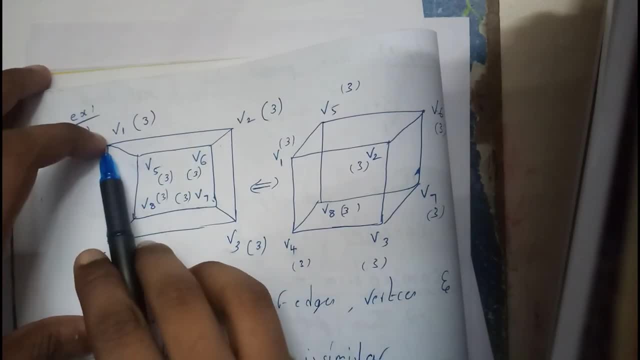 you And just write down the degree at each Degree is nothing but the number of vertices. So this is something like a cuboid. This is also a cuboid. This is also a cuboid. And just write down the degree at each Degree is nothing but the number of edges that passes. 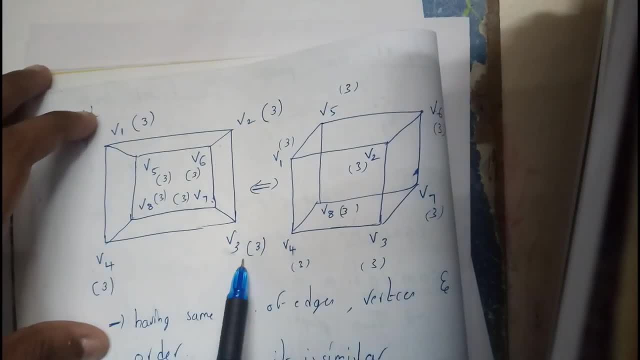 through that vertex V1,, there are 3. V2,, 3. V3,, 3. V4,, 3. V5,, 3. V6,, 3. V7,, 3. V8, also. 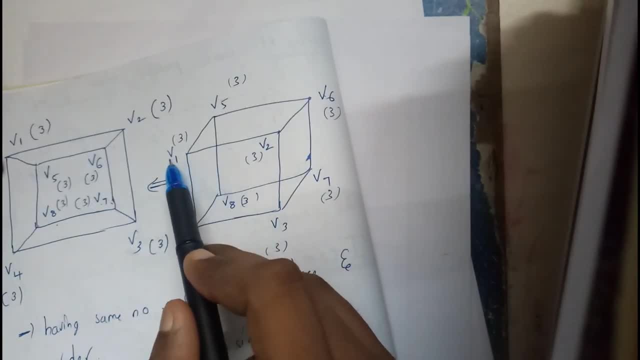 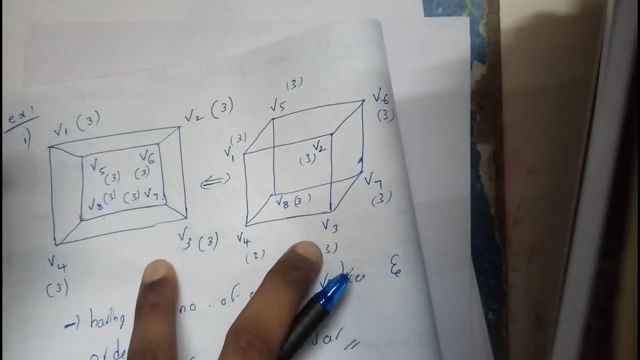 3. Even though here also we are having for V1, 3. V2, V3.. All are similar, Whereas, whenever you want to, For the first case all the vertices are same, All the degrees are same. So now, 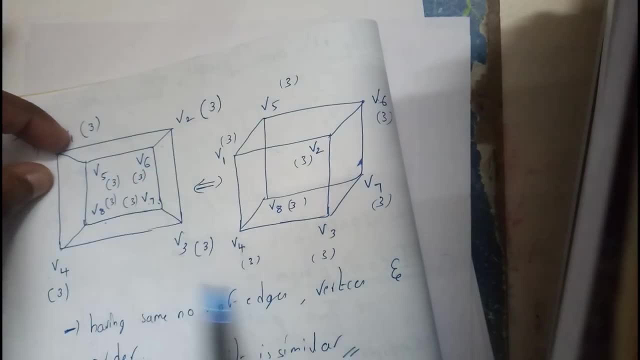 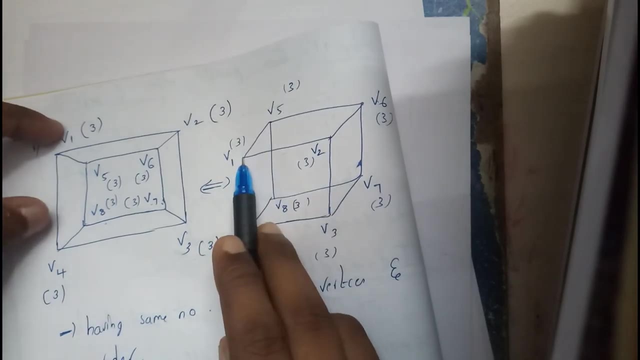 let's come to edges. Here we are having V1, 2. V2.. Here we are not having V1 to V2.. Okay, we are having V1 to V2.. V1 to V5, we are having. 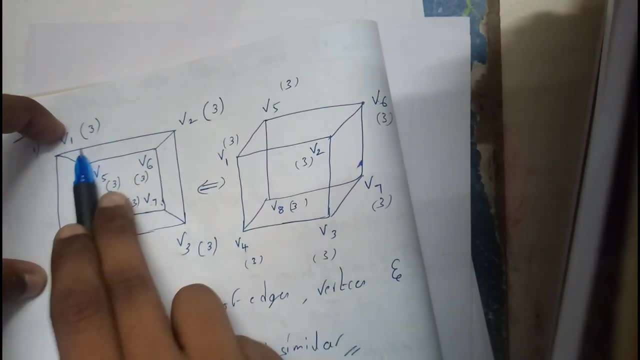 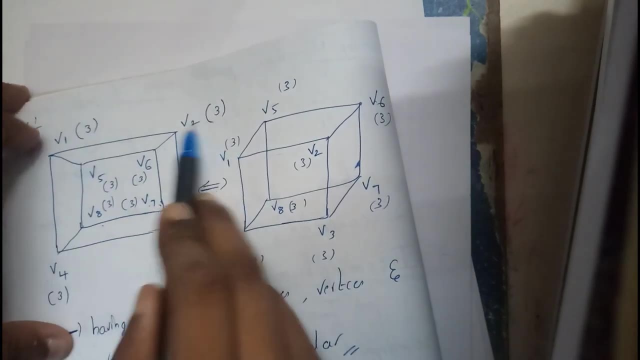 V1 to V5, we are having. V1 to V4, we are having. Yes, It is isomorphic. Everything is similar. If you want, you can check step by step. V1 is done, V2 to V1.. V2 to V1.. V2. 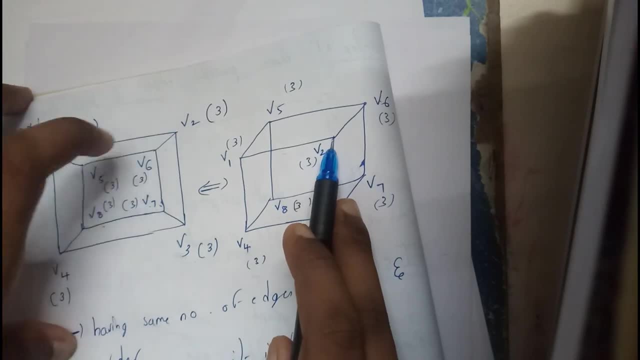 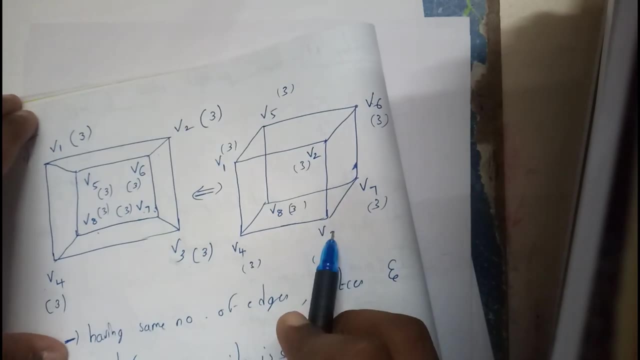 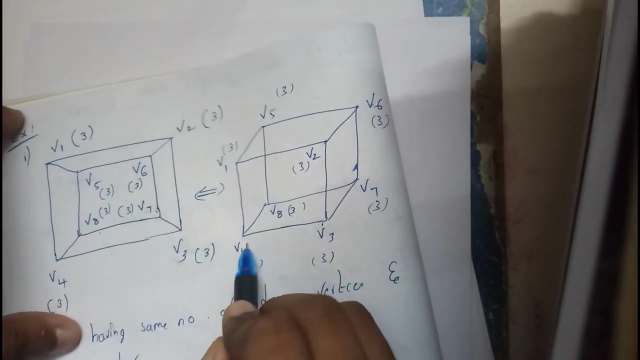 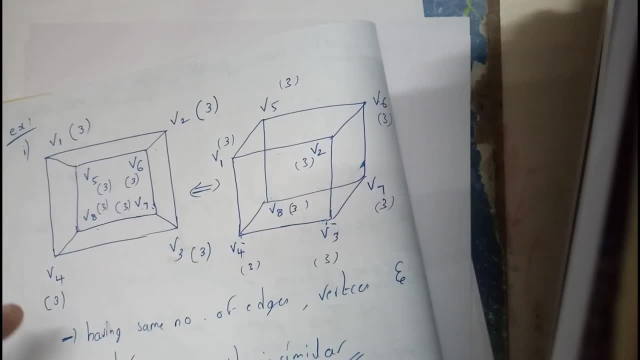 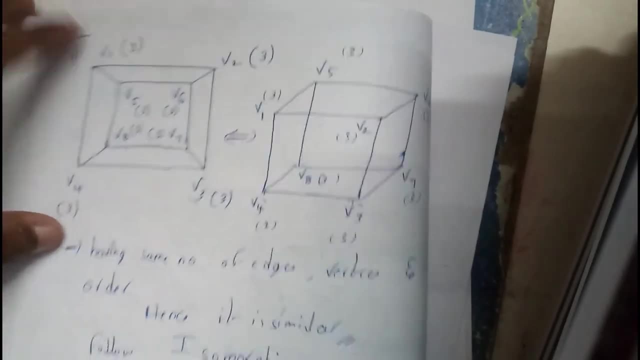 V3.. Yes, This is an isomorphic graph, As the number of edges are same and the map from same vertices. Hence the following two are isomorphic. Thanks for watching the video, guys. Thanks Bye.